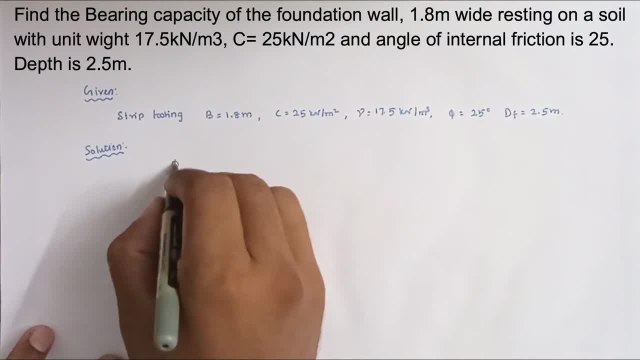 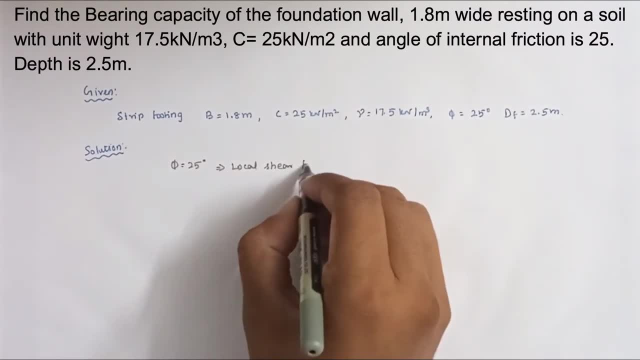 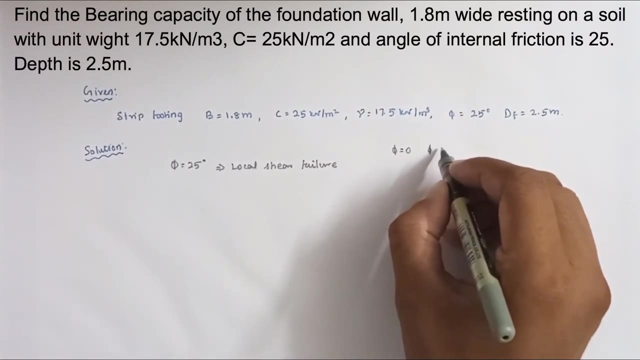 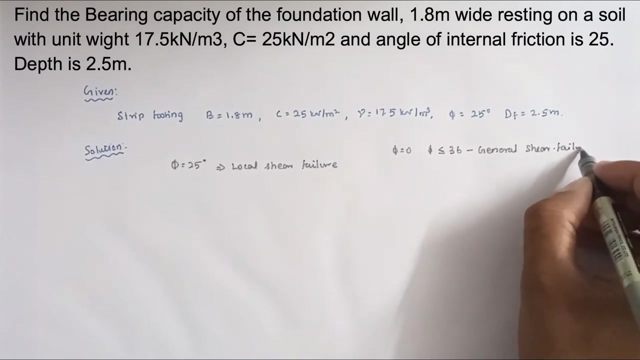 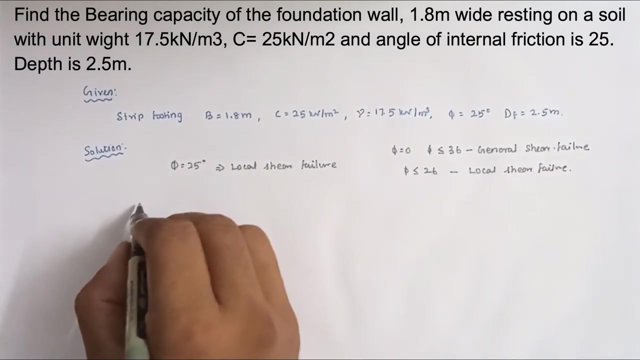 find out the bearing capacity. so now, first, 5 is equal to 25. so this is local shear failure. so we know, 5 equal to 0 or 5 is more than 36, there is general shear failure. so below the 5 is equal to below 26, this local shear failure. ok, so now the formula qn is equal. 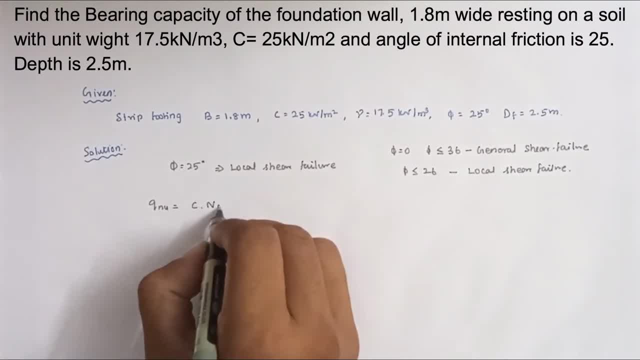 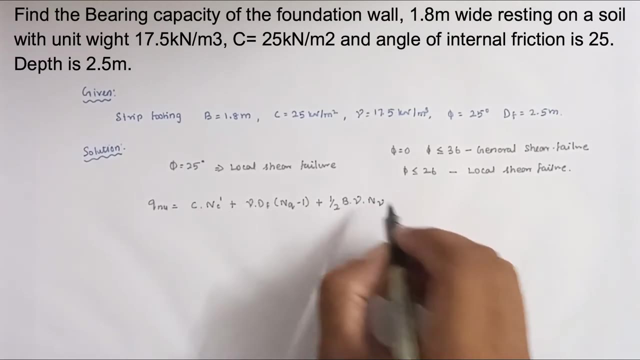 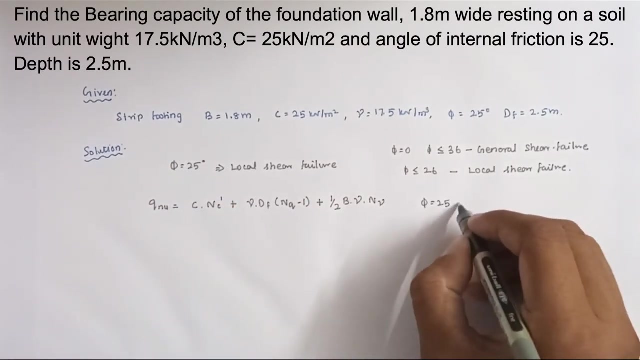 to tesla. formula qn is equal to c into nc, dash plus gamma into df, into nq, minus 1, again plus off into b, into gamma, into n gamma. so this is the formula for bearing capacity for strip footing. so for 5 is equal to 25, the nc, nq, n, gamma values taken from the bearing capacity table. 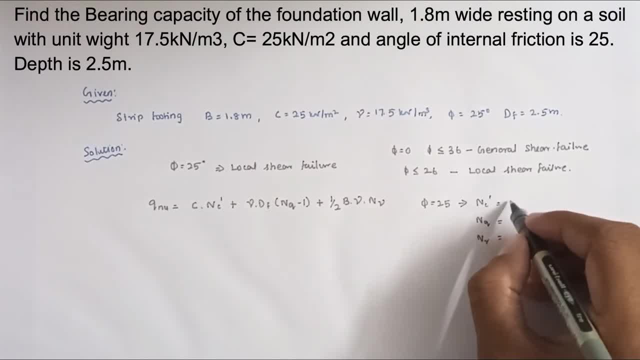 so this values taken from the bearing capacity table and the nc, nq. nq is equal to 25, so this values taken from the bearing capacity table and this values taken from the bearing capacity table. so nc dash is equal to 14.8, nq dash equal to 5.6 and n gamma dash is equal to 3.2. so 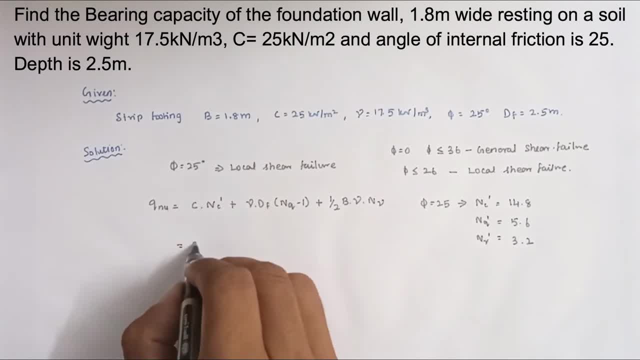 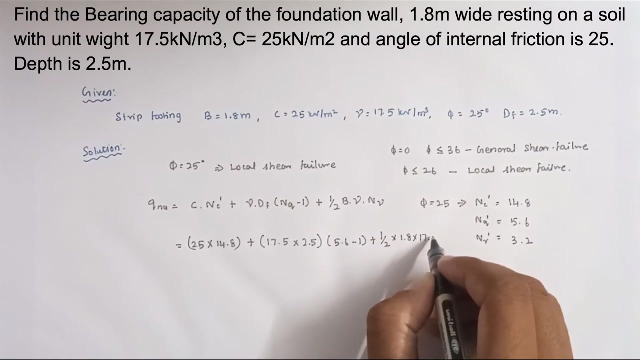 we can substitute all the values over here. so c is equal to 25 into nc value is 14.8, again plus gamma value is 17.5. into so depth this equal to 2.5 meter. so into nq values 5.6 minus 1 plus off into so b value is 1.8 into gamma 17 point 17.5. into n gamma values 3.2. 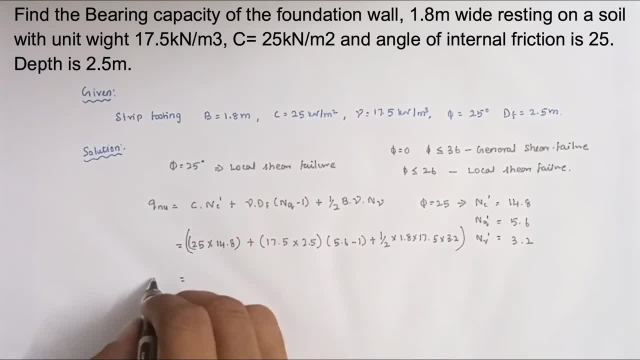 okay, so we can solve the evo equation. so n q nu is equal to. we got the value of 6 to 1.65 kilo newton per meter square. okay, so again. uh, we'll see q n s, so net safe bearing capacity. so